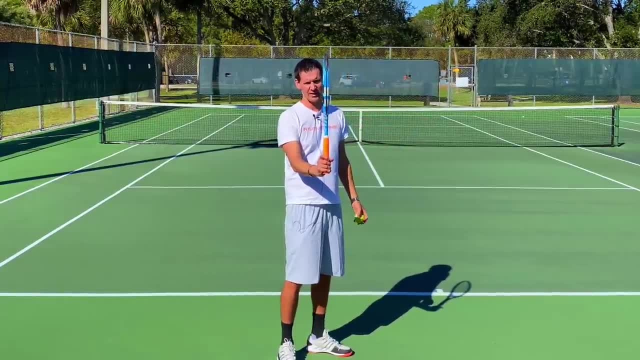 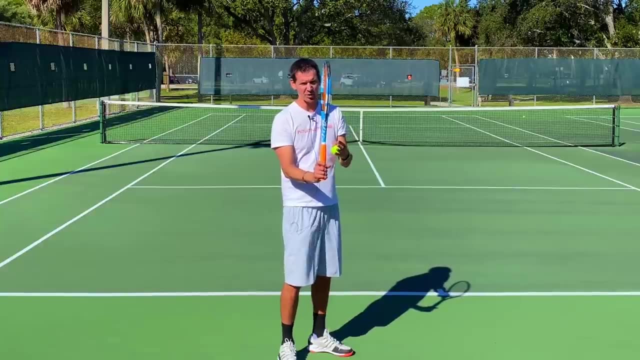 too straight down. So, with this angle of the racket, face a neutral position. there are certain ways to get more height on your kicker, but it's not by trying to hit up on the ball, And many players believe that you should try to hit up on your kick serve in order to get height and 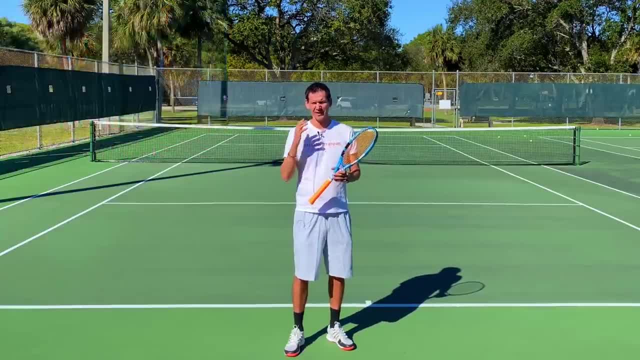 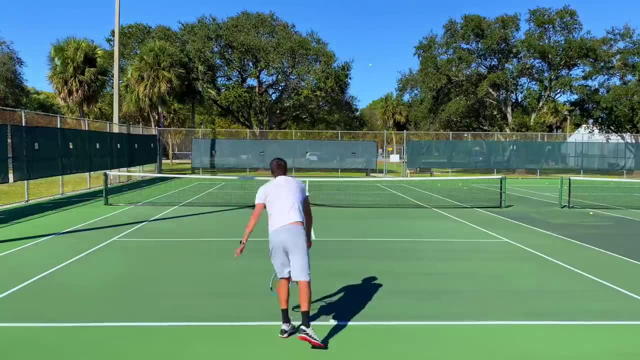 it's absolutely not what you're supposed to do, because if you try to hit up and your kick serve, the ball will go over the fence. Now let me demonstrate. So if I hit up on this served ball, it's not going to be able to go inside the box, So you should never try to consciously. 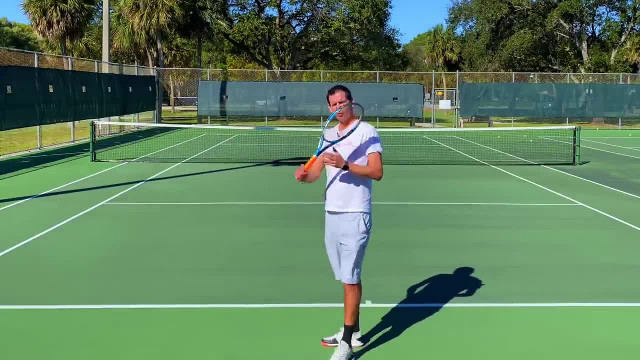 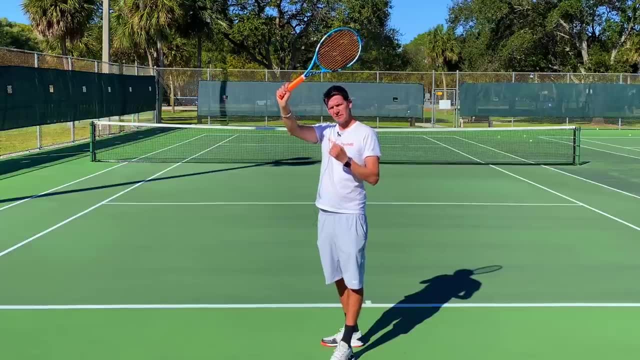 go up. See, what happens on a kick serve is that we're going to have a more angled position of the racket head at the moment of contact- And now any serve in tennis- once contact is made, the entire system is starting to move downward, and it's also true for the kick serve. So the hand will go down. 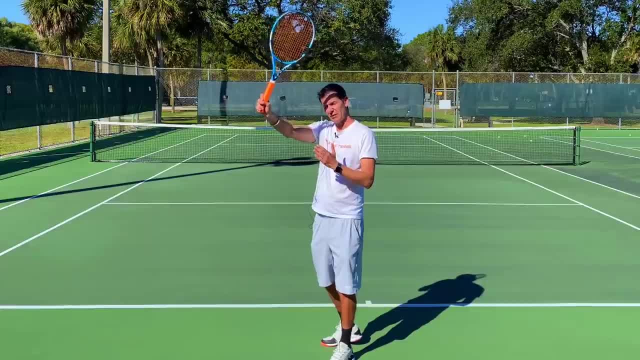 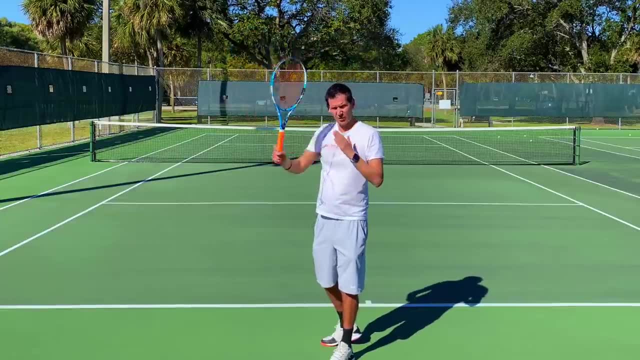 while the racket head will go up Up in this way. so this is what creates the kick. So the angle position of the racket face is going to straighten out while the hand is going down, and this is why the trajectory of a kick serve is always down. 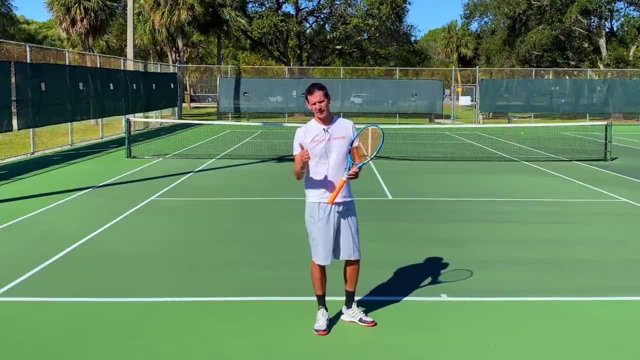 Now the position of the racket face at contact on any serve, whether it's the flat, the slice or the kick, is going to be neutral. This is how the racket is positioned on all serves and this is going to be the most important thing in terms of the ball's trajectory, if you execute the fundamentals. 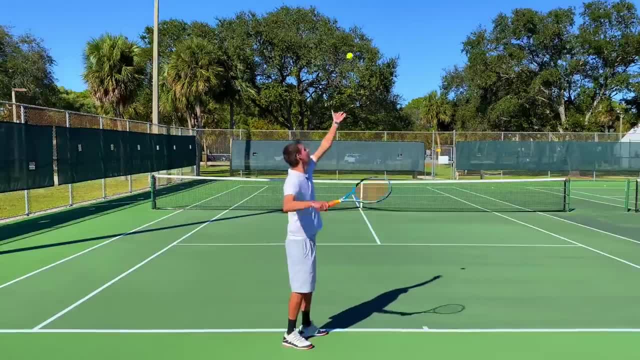 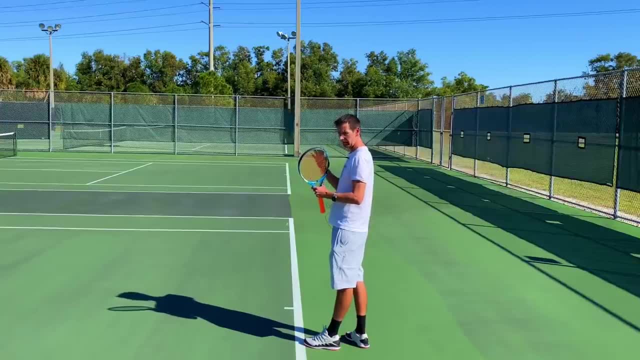 correctly. So what happens with a lot of players? they try to get kick. they actually throw the ball behind them and naturally, when the ball is way behind the body, the racket will open up if the ball is tossed behind your body. So we need to toss the ball a little bit more in front so that 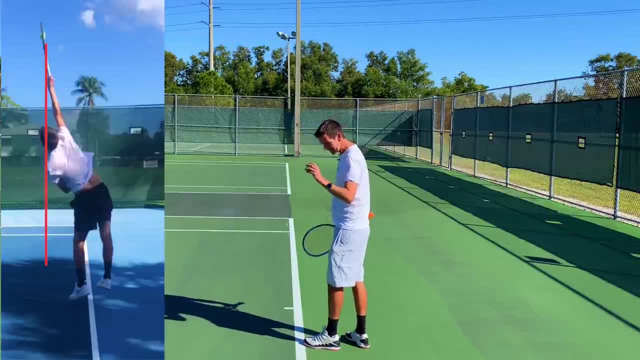 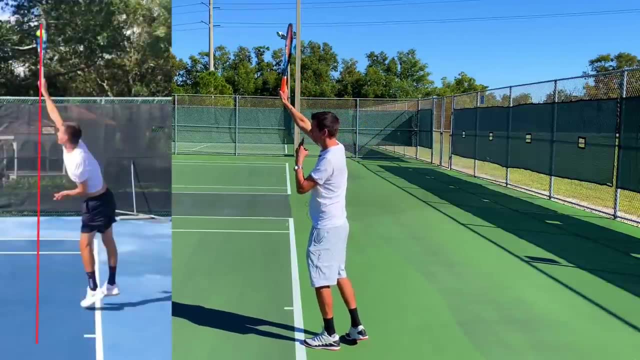 we can strike the kick serve right above our head, and this is going to require that we toss the ball at least at the level of the baseline. Now the flat and the slice serve have a contact that's far more in front, so it's going to occur. 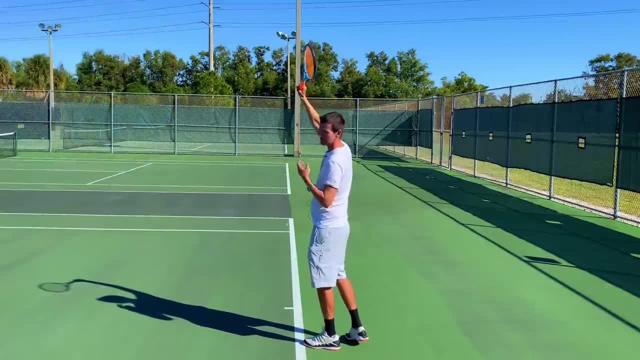 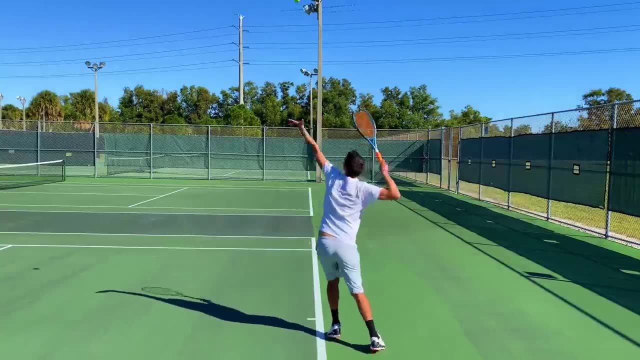 while the kick serve is struck right above the head, and this is very important when it comes to the height of the serve. So what's going to happen is that we strike the ball way in front of the body. like this, This serve is going to have less height than a serve that's struck above our head. 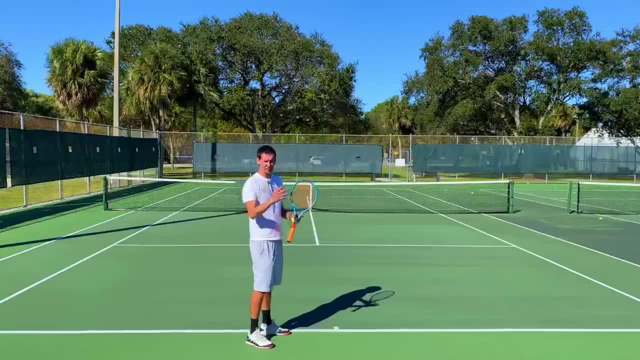 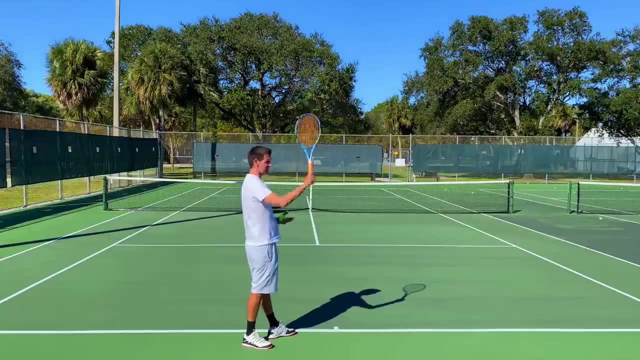 right along the baseline And take a look from this angle. so, on this serve, I'm going to throw the ball way ahead of me, in front of the baseline, and the contact is going to occur in front of my head, and you pay attention to the trajectory of the serve. 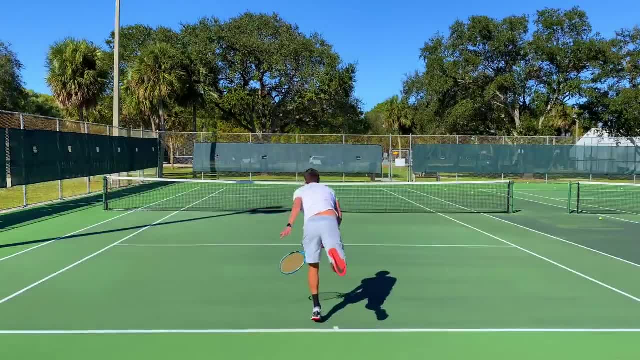 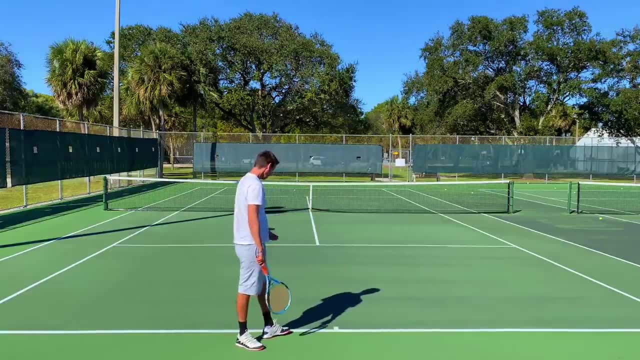 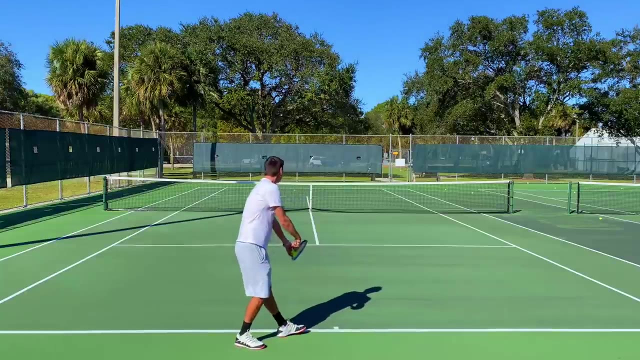 You can see here that serve went very low over the net and also it didn't bounce very high on the other side. so now I'm going to throw the ball along the baseline and you pay attention to the trajectory and the height of the ball. You can see here that the ball cleared the net at a much higher level and it also had a much higher. 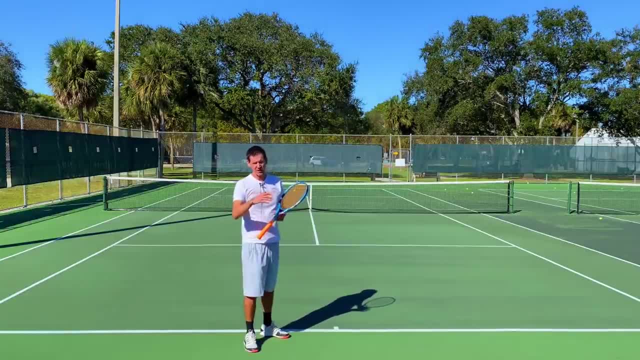 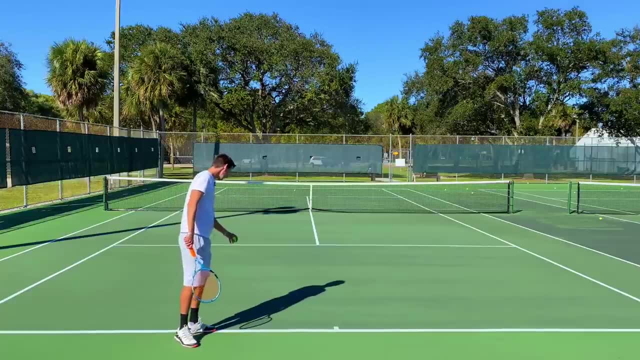 bounce once it landed on the other side. If you watch professional kick serves, you will notice that even on the kick serve there's a little bit of a difference in your get on the ball kicker that throw the ball way inside the baseline. and this is where the topic of height and kick. 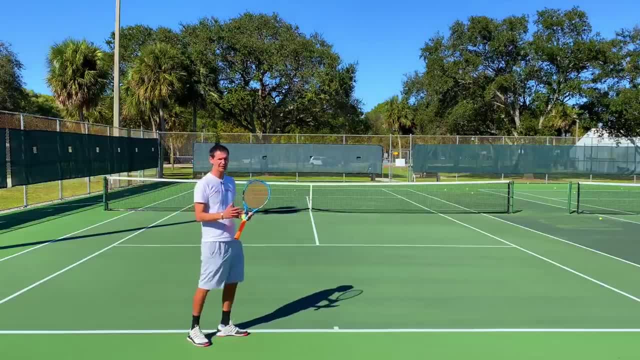 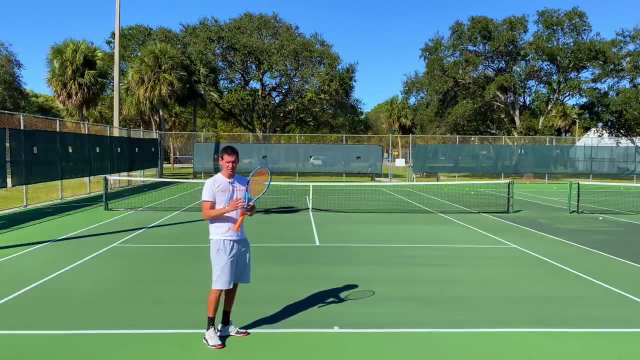 serves gets a little complex. So the reason why professional players, even on the kicker, throw the ball in front is that they want to generate forward momentum. Forward momentum is a big power source on the serve and many recreational players do not serve a kick serve with forward momentum. They 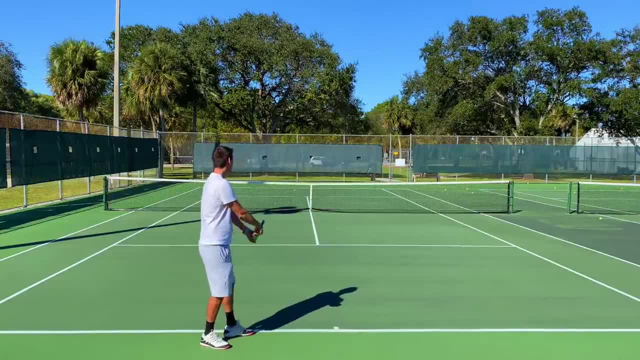 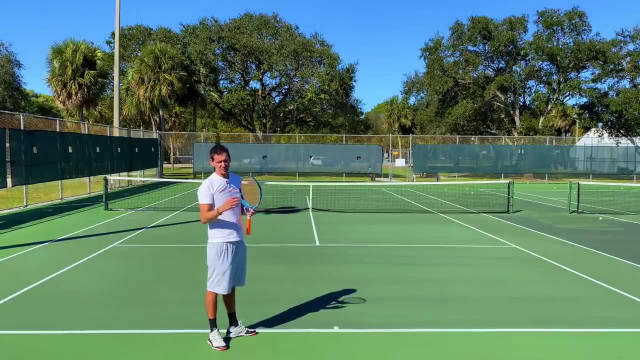 basically be stationary. So when you're stationary and kicking the ball, yes, you will be able to get height on the ball and you will be able to kick it, but you will never get the same speed that you could get if you executed the serve with forward momentum. So what happens, unfortunately, is that 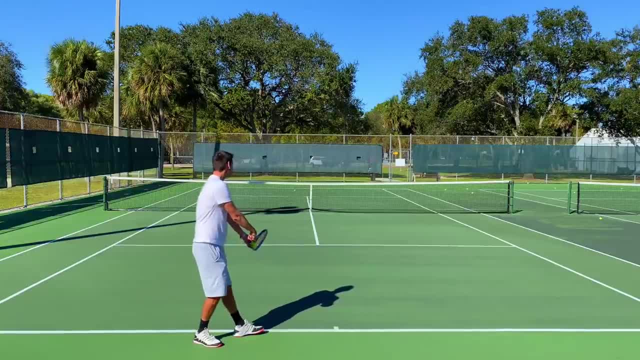 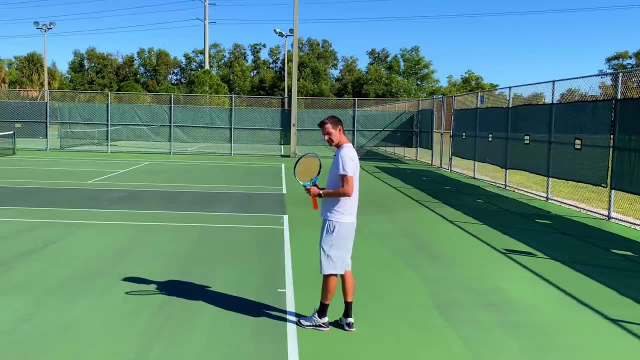 when you throw the ball in front and then execute a kicker. now you're going to lose some of that height. And the reason for that is quite simple: If we're in a stationary position and we extend the arm fully on the kick serve, we're going to get more height. In other words, we're going to contact the 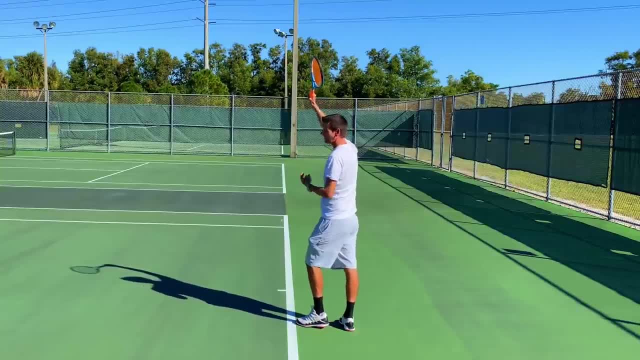 ball at a higher point than if we throw the ball at a higher point than if we throw the ball at a higher point. So we're going to throw it in front and then lean forward. This will lower the contact points. Let me show you from this angle so you can see the trajectory of the kick serve. So on this one, 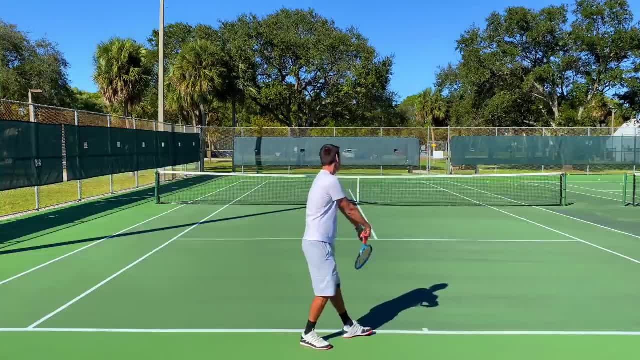 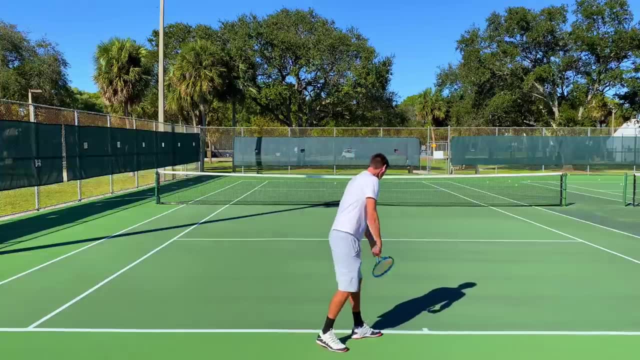 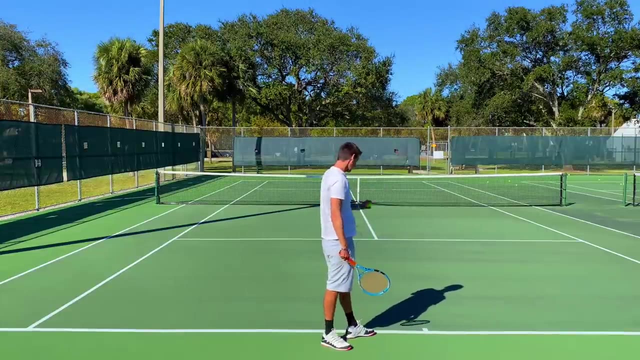 I'm going to throw the ball in front and kick it. You take a look at the trajectory, See there and now I'm not going to lean in, I'm going to be stationary and I'm going to kick it. You can see there is significantly more height on the second one. Let me try it again. 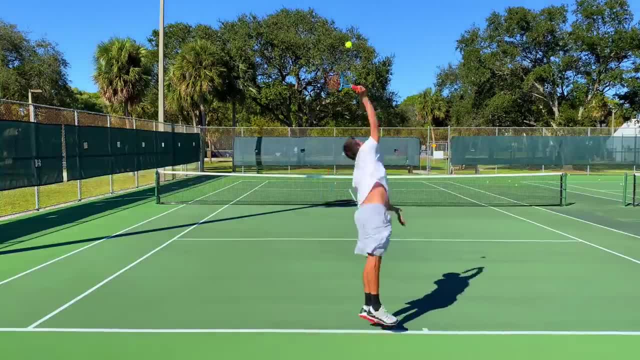 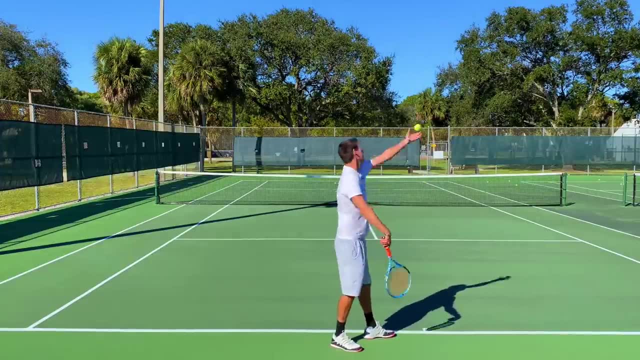 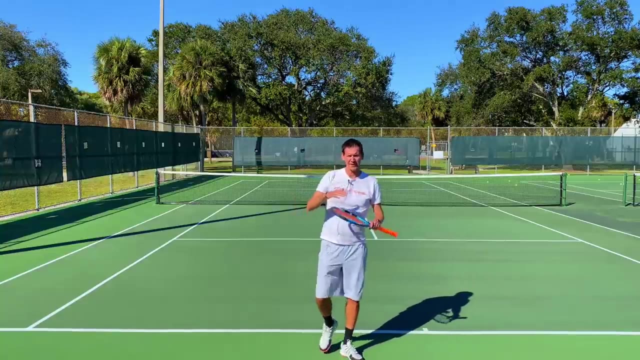 This one, I'm going to throw it in front and kick it, And on the second one, I'm going to be stationary and hit a kick serve. You can see that I missed that one, but you can see that the ball is clear net much higher on the stationary serve. So what does this mean? Well, I definitely don't want you to lose. 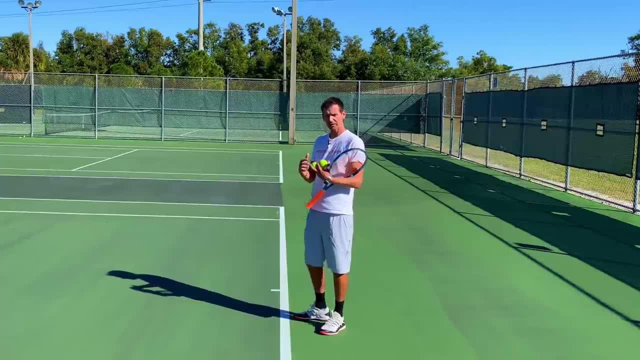 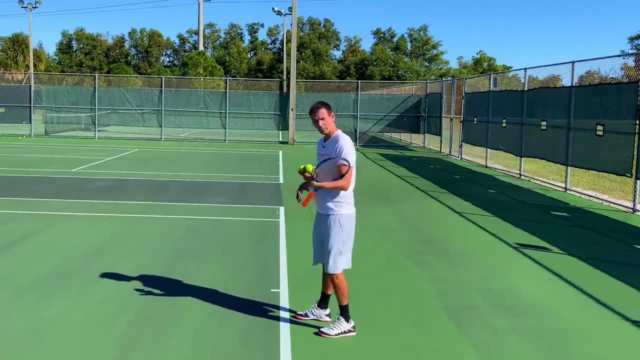 out on the forward momentum because it can come in very handy. See, a lot of players get a little bit tight on their kick serve because they use it as a second serve. So when you execute forward momentum, going forward with the body will often be a little bit more difficult. So you're going to want to 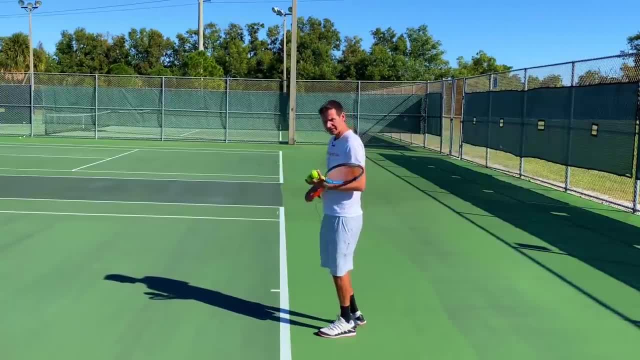 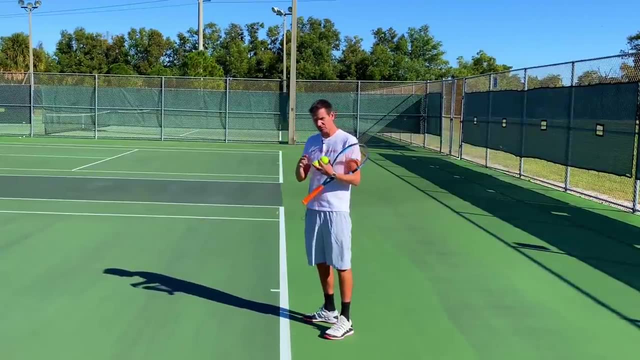 try to find ways to extend the body time during the kick serve and help the ball go over the net. In addition to that, it is a fantastic power source that I definitely don't want you to lose out on. So how do we get forward momentum and height on a kick serve? Well, there is a way and we can learn. 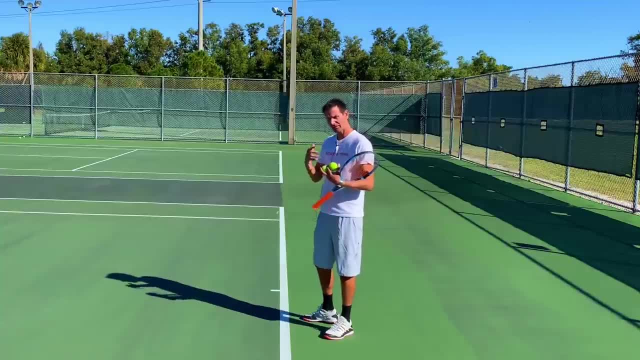 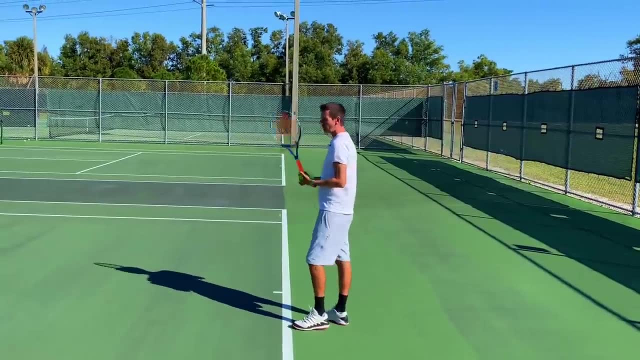 from the great Stefan Edberg, who had one of the most amazing kick serves of all time, And what Stefan used to do was he used to throw the ball in front, but he would get his body underneath the ball, So, in other words, he would not allow the contact to get ahead of him, because this will lower. 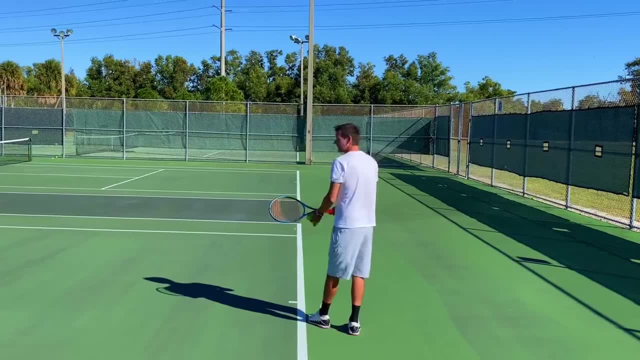 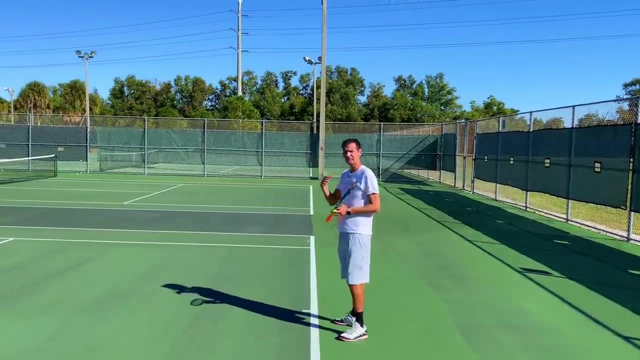 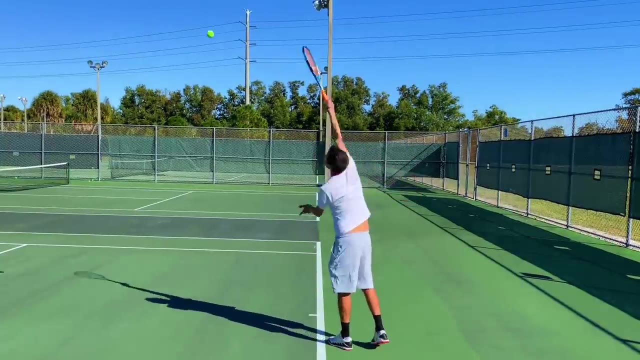 the trajectory of the kick. serve severely would throw the ball slightly in front and then get his body underneath the ball, and so when you do this, this will make the contact much higher. it will almost make it like a stationary serve. So on a stationary serve we get a much higher contact point, as I previously discussed. Now, if we can, 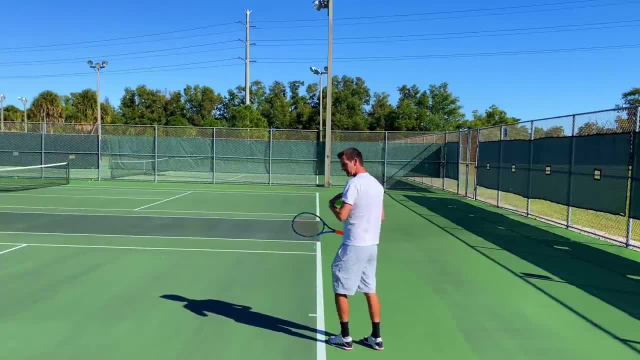 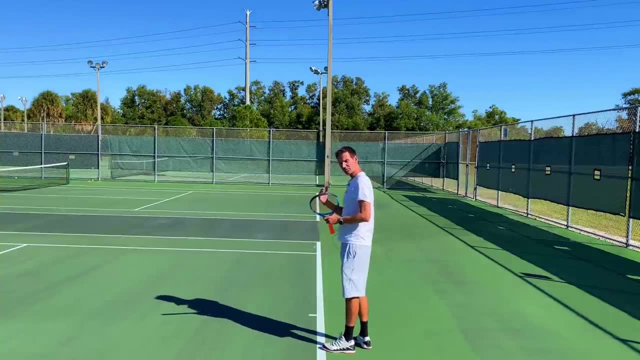 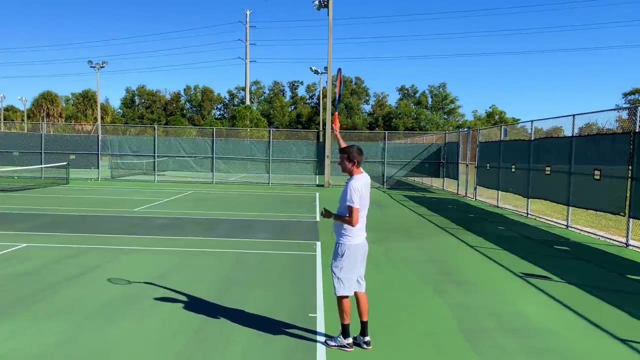 get our body to be in that same position inside the court like this: we slightly lean forward, but we stay more upright with the torso. we don't quite lean as much as we would on a flat serve and we keep our body upright and then go forward. now we can get the same type of height that we get on a 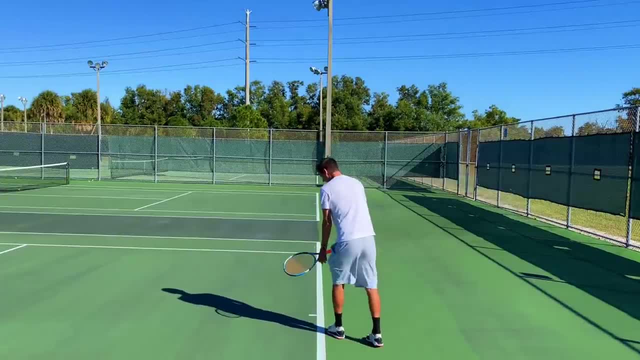 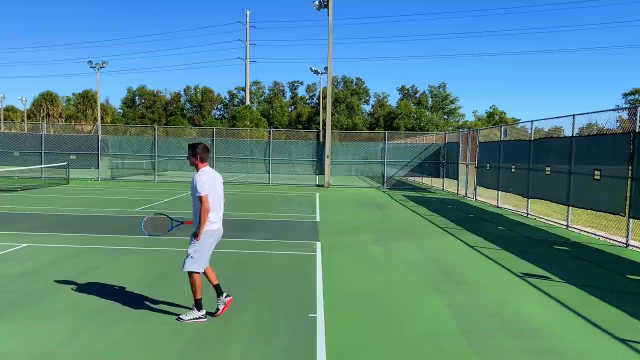 stationary serve. So, guys, let me show you. I'm going to do the Stefan Edberg kick. I'm going to get my body underneath the ball and keep it upright, and this works fantastically well. Alright, guys, let me show you from this angle so you can see the trajectory of the serve. So I'm going to do the. 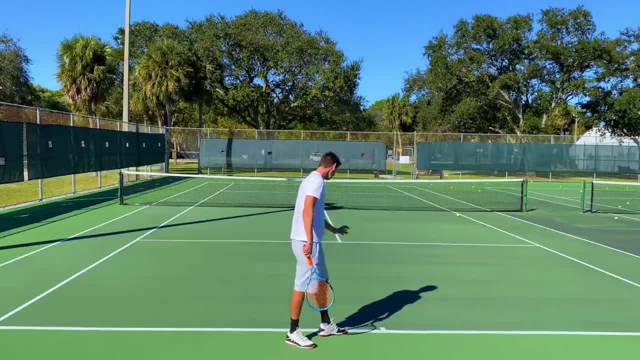 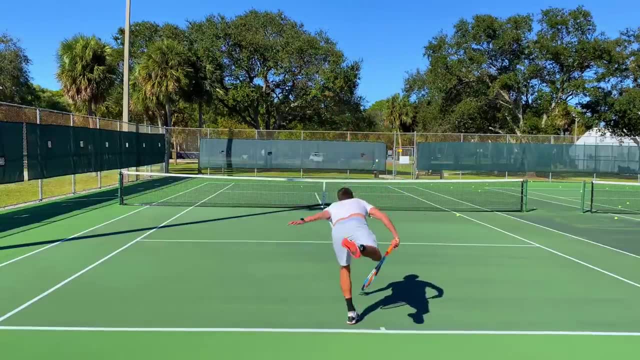 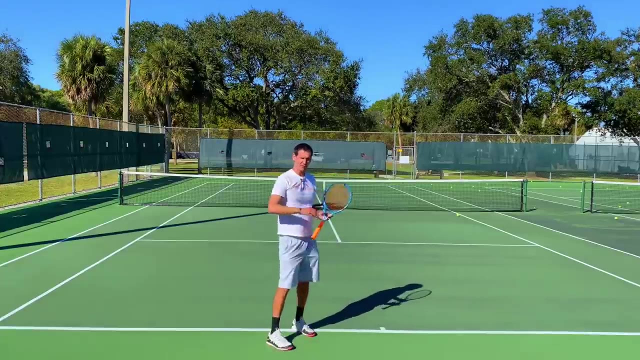 Stefan Edberg technique. I'm going to throw the ball slightly in front, but I'm going to get my body underneath the ball and keep it quite upright. You can see there the ball has significantly more height compared to a serve where I'm simply leaning forward like I would on a flat serve. Take a look, so if I don't get my body.